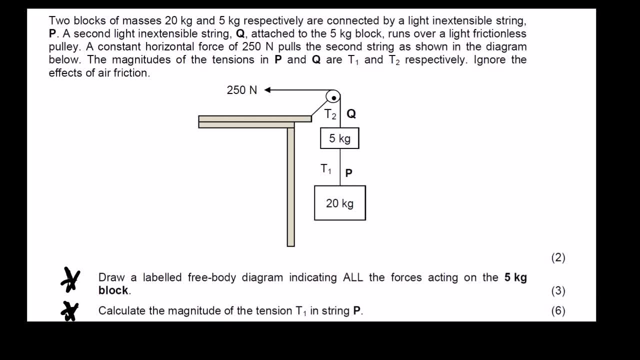 respectively, are connected by a light inextensible string P. a second light inextensible string Q attached to the 5 kg block runs over a light frictionless pulley. A constant horizontal force of 250 newtons pulls the second string as shown in the diagram below. The magnitudes of tension: tensions in P and Q are T1 and T2. 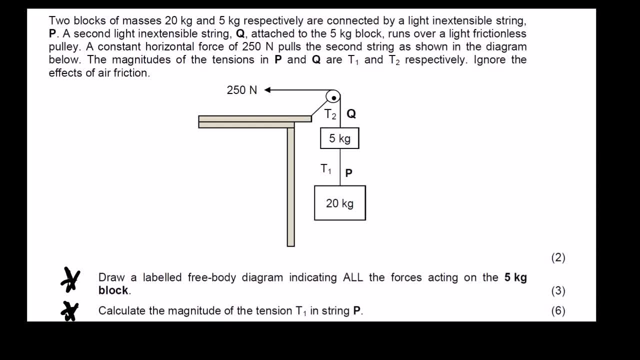 respectively: Ignore the effects of friction. There is a lesson video whereby we focus on the basics of this calculation. This question is based on Newton's laws and applications of Newton's laws, So just make sure you watch that lesson video if you get lost throughout this lesson video. So here: 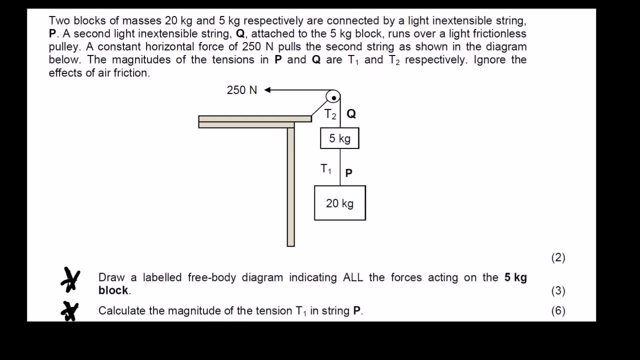 we can see, we have these two diagrams: The first one is 5 kg, the second one is 20 kg, and then we have T1 and T2.. And then we also have force applied on T2.. So the first question: you see and draw a. 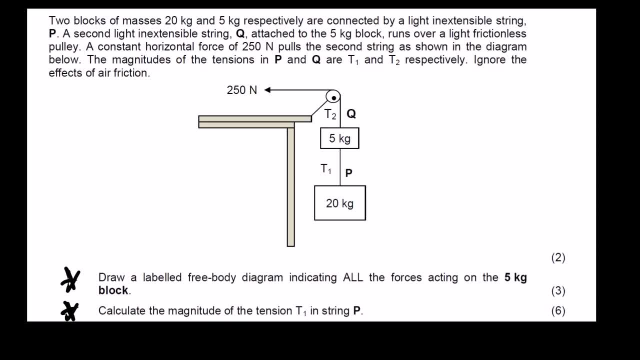 labeled free body diagram indicating all the forces acting on a 5 kg block. Now, to answer this question, I will just add a bit. We are going to draw free body diagrams for both of these objects. So for 5 kg, remember we represent an object using a dot. Looking at the force diagram of this block, we can see- we 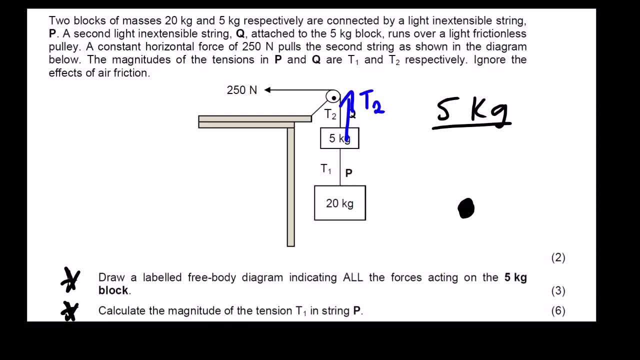 have T2- this direction, We have T1- this direction and we have FG. So basically our free body diagram will be like this. So the free body diagram it will be T2, T1 and then we have weight or we can say FG. 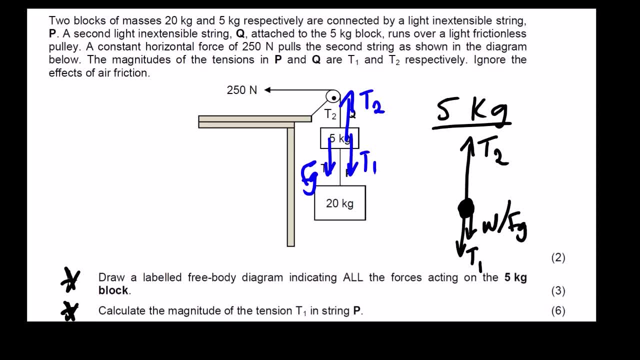 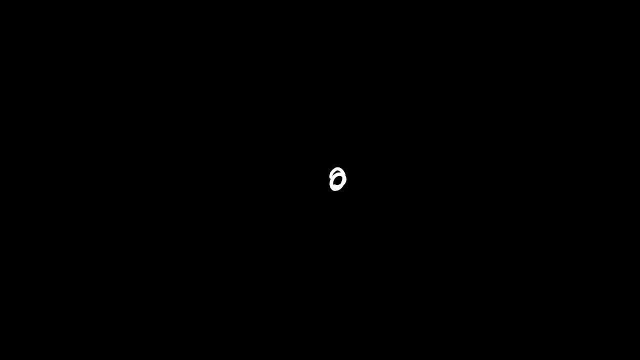 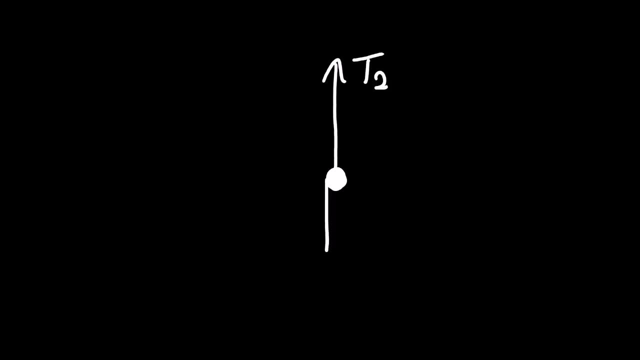 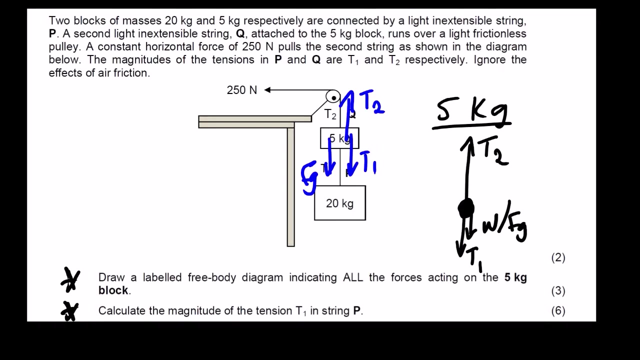 Let's actually draw this. What we can see is a dot representing an object. So we have T2.. We have T1., Then we have weight. So this is the free body diagram, And the mark allocation for this question will actually guide us on how many forces are. 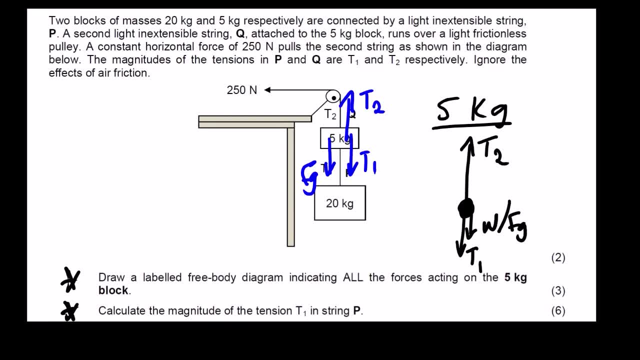 acting on this block. Since it's 3 marks, just know that we are going to have three forces. so this is actually our free body diagram. now let us look at the 20 kg block. so it's a dot, and then we have t1 and weight. so you only have two forces acting on this block. 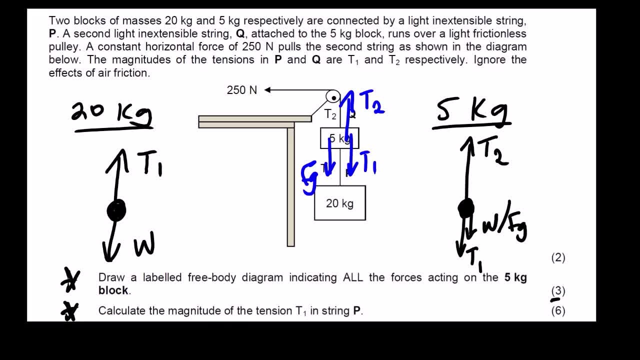 now going to our next question. it's saying: calculate the magnitude of tension t1 in string p. so we are looking for- we are actually looking for- this t1 and looking at the micro location you can see that our steps will be a bit longer, but it seems like. 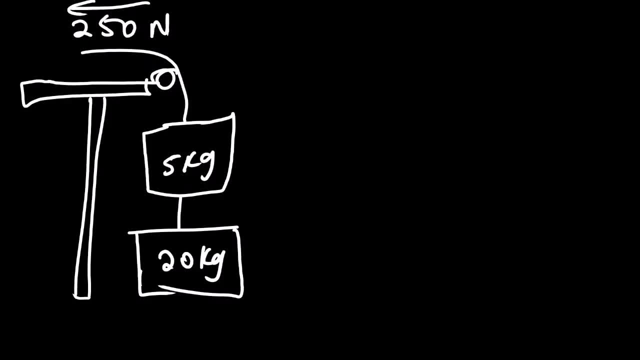 simple. it's not difficult. we need to understand something now. if we apply 250 newtons this direction, it means the whole system will go up. so since the displacement of the whole system is up, i'm going to consider up as positive, down as negative. it means all the. 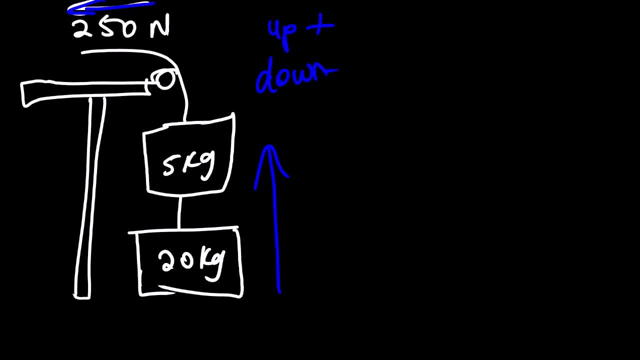 forces facing up will be positive, all the forces facing down will be negative. and then we also need to take note that we are actually applying 250 newtons on t2, so we can say t2 is equal to force applied. and then we are looking for t1. 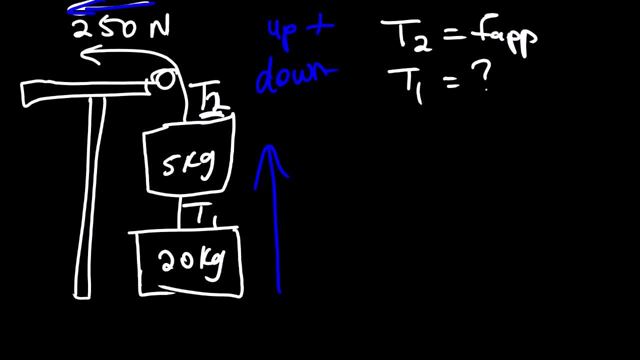 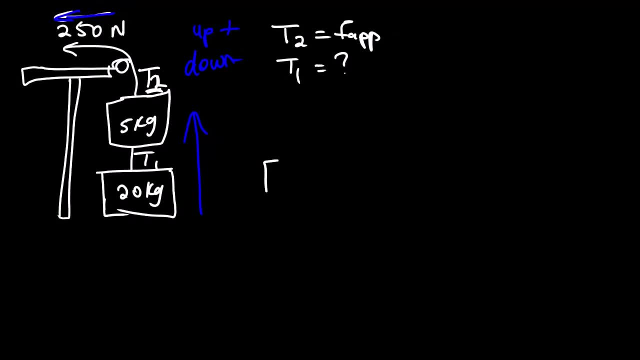 we need to generate equations. so we have f net is equals to ma. we are actually focusing on 5 kg block. then we said how many forces are acting on 5 kg block? remember, our free body diagram is like this: t1 and weight. so we are actually focusing on 5 kg block. and then we said how many forces are acting on 5 kg block? 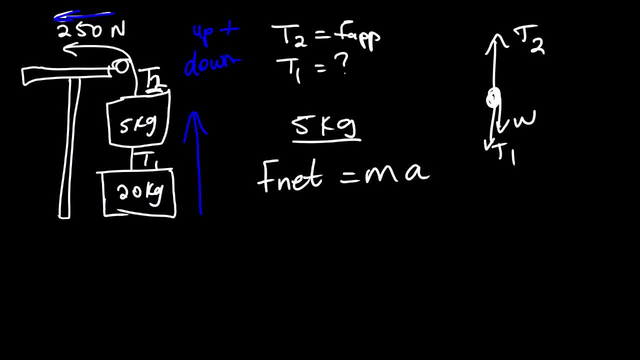 so we can see that we have three forces. how many forces are facing up? we have only one force, which is t2, so our t2 will be positive plus, remember, f- net is the sum of all forces acting on the block. then we have another force, which is t1, so it will be t1. since it's facing down, it's negative. 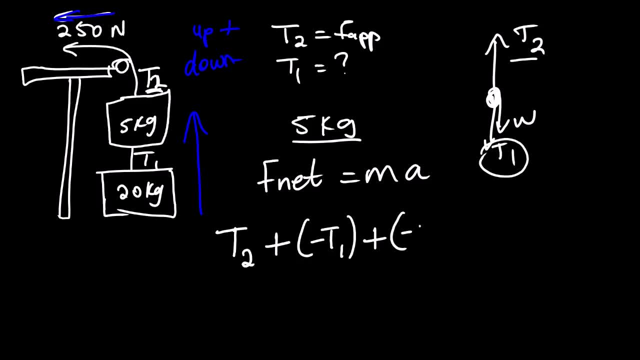 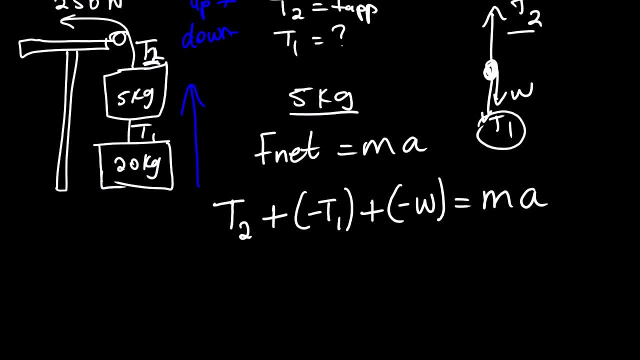 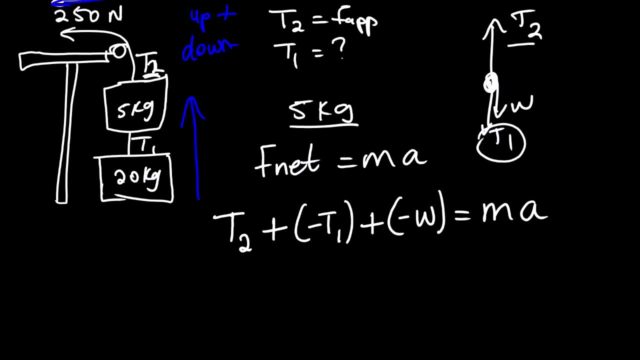 plus we have another force, which is weight. it's equals to ma. from here, since we said, t2 is the same as force applied, since we're applying force on tension 2. so t2 is 250 newtons minus t1. and then remember weight, weight it's. 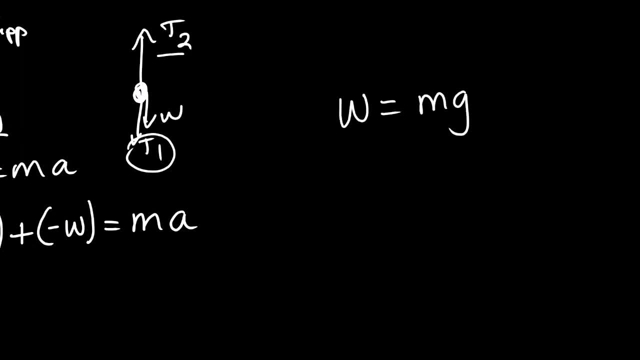 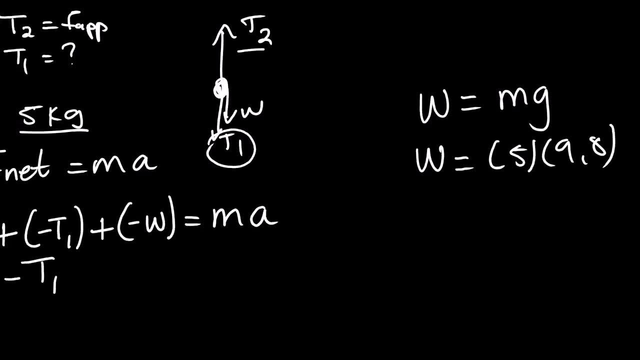 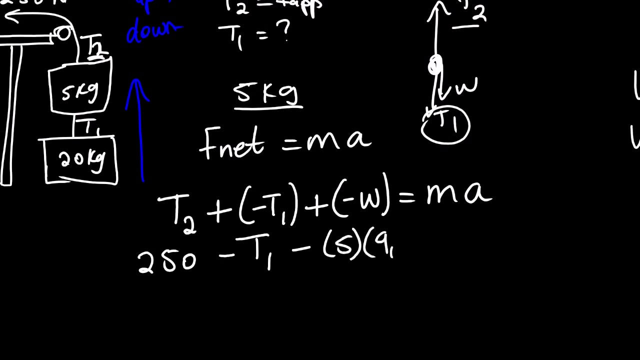 fg weight, it's equals to mg. so, since we have the mass, the mass is 5 multiplied by 9.8 meters per second. so we can substitute here: 5 multiplied by 9.8, it's equals to the mass. you are still focusing on the 5 kg block, so it's 5a. 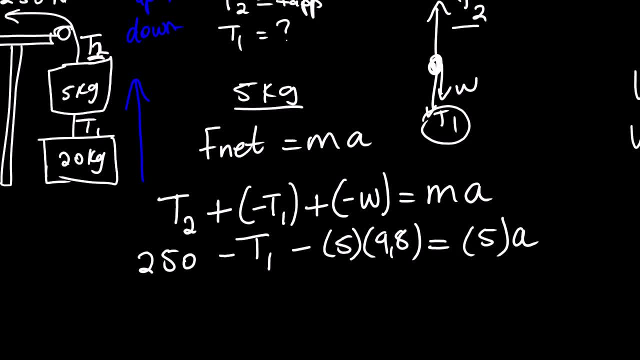 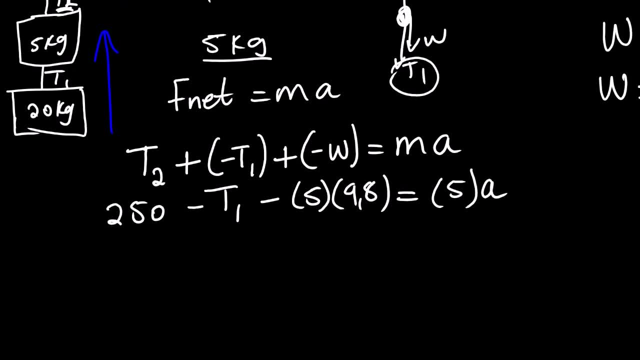 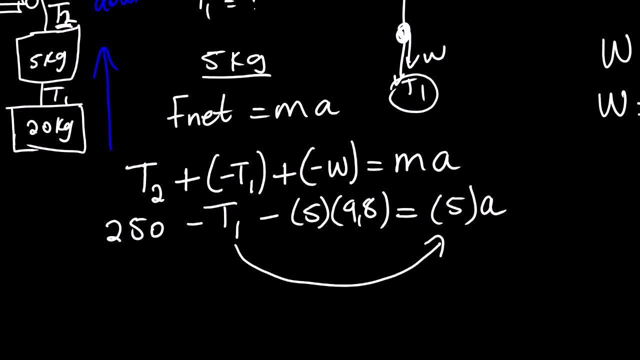 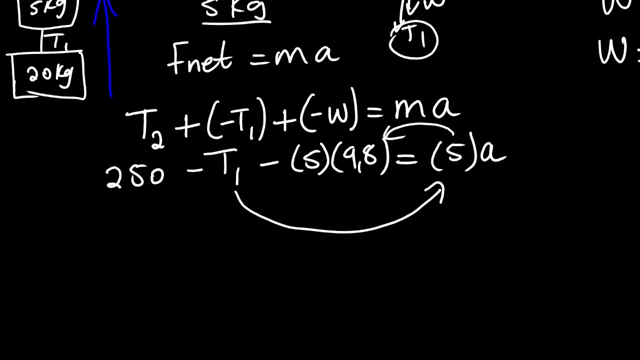 remember, we don't know the acceleration of the system. we are looking for t2, so we need to make t2 the subject of the formula. so what we can do, we can transpose t to this side and take 5a that side, such that we have something like this: t1, it's equals to 250 minus. 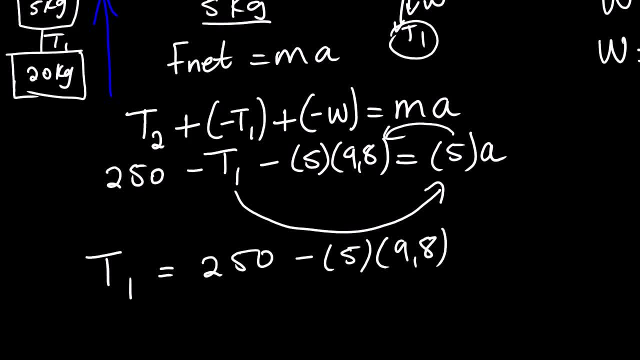 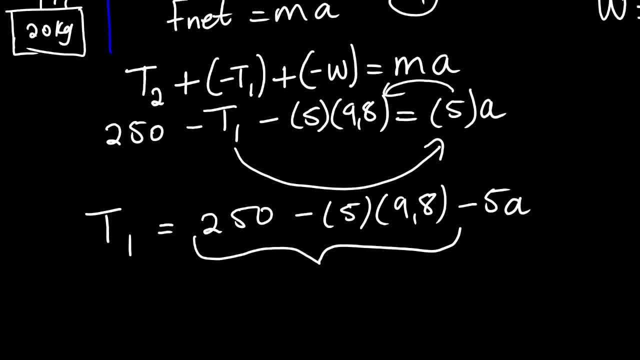 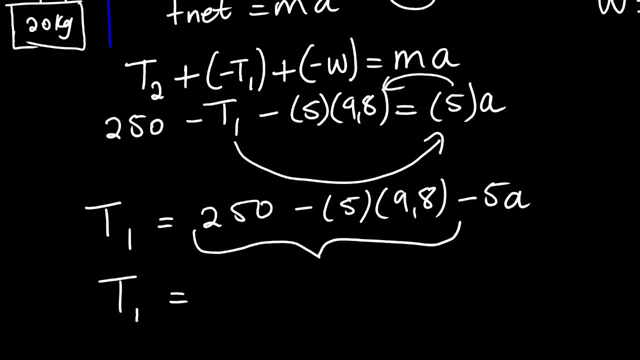 t2 minus t2, 9.8 minus 5a. so we can quickly simplify this. so 250 minus 5, 5 multiplied by 9.8, is 201 minus 5a. so we equate this as equation 1. we generated this equation from 5 kg block. 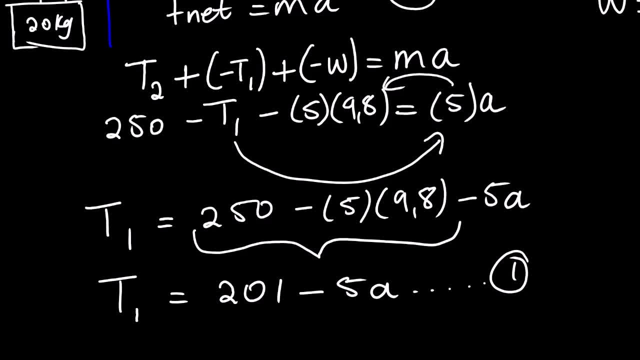 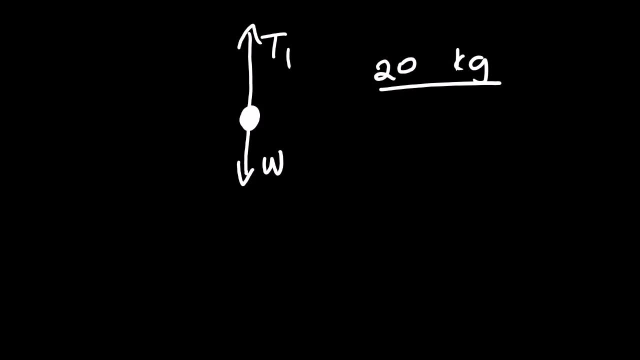 now we need to proceed and generate equation number two from the 20 kg block. for the 20 kg block, we have two forces acting on it, so we need to start with F. net is equals to ma. now how many forces are actually on it? we have two forces now. t1 would be positive. 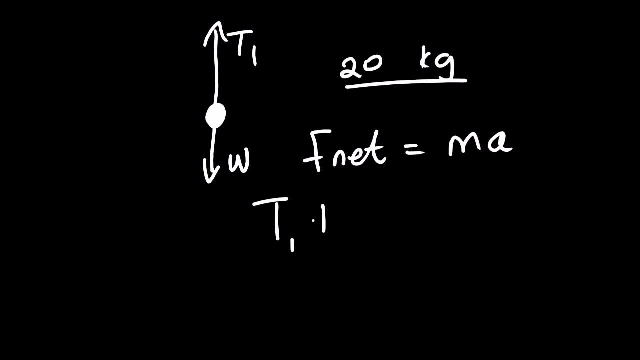 since it's going up, it's facing up, plus negative, and then it's ma. now we have t1 minus M G, it's equals to M e. and then t1 is equals to 20 kg, actually negative, negative. 20 kg multiplied by 9.8 it's equals to 20. 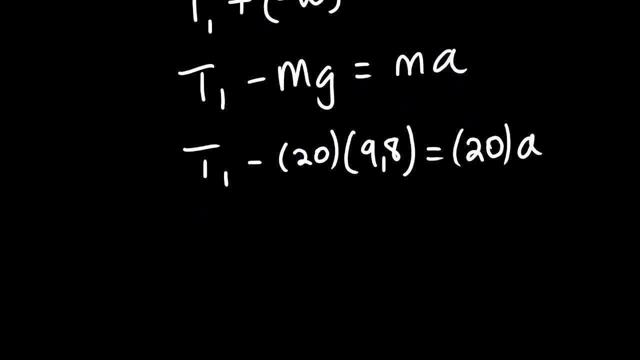 multiplied by 8, so we can take this to the other side. so we have T: 1, it's equals to 20, 20 a plus. let us quickly simplify this: 20 multiplied by 9.8, it's 1, 9, 6. so this is equation 2. now, as you can see equation 1 in equation 2, T is: 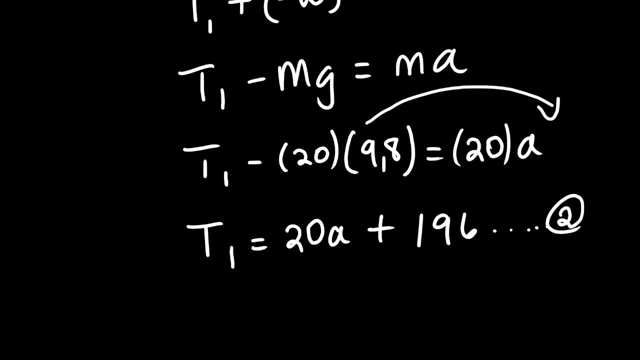 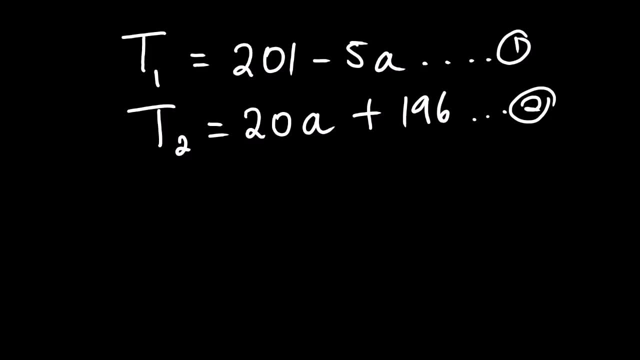 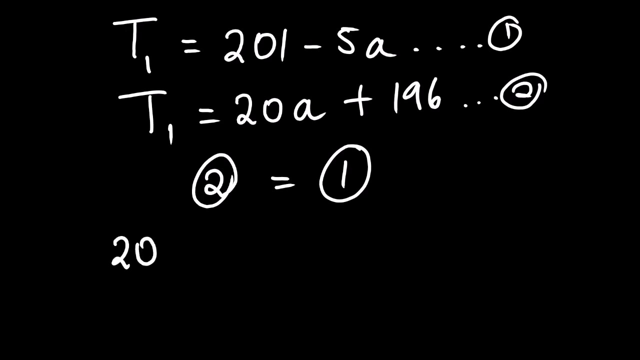 the subject of the formula. we can equate the two equations and solve for the unknown, which is the acceleration. these are our equation. so now it's actually T: 1, so we can equate the two equations since T is the subject of the formula. so equation 2: it's equals to equation 1. then we have 2, 0 a plus. 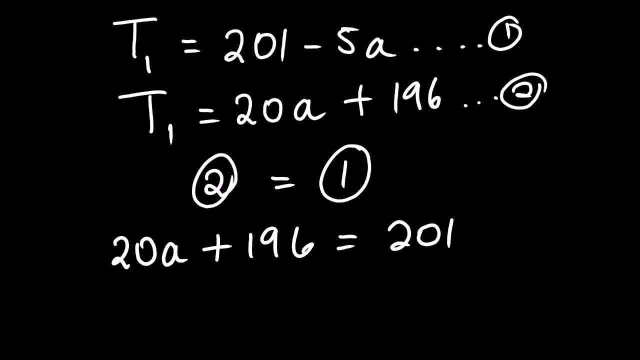 20 1, 9, 6 is equals to 201 minus 5 a. then we solve him for a. we take this to the other side and then we bring this one to this side, so you are going to have 20 a plus 5. a is equals to 1 negative 196 plus 2. so 20 a plus five- it's actually 5g- is equals to 906. localization equal to 20mh per second. plus 5 a minus 5 a equals 20.94 is equal to 10. they equal to 20.. Element of minus 196 plus 20 A. we take this to the other side, then we bring this one to the side, so you are going to have 20 a plus 5a is equals to 192 angular. 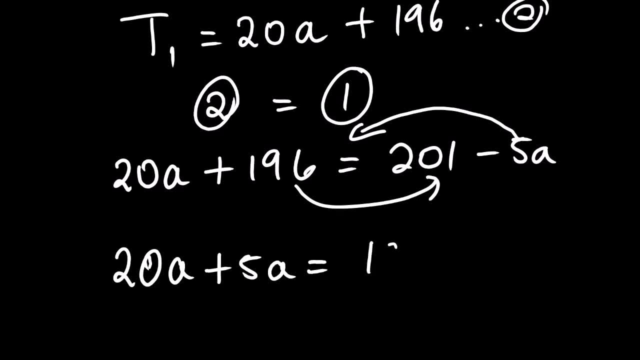 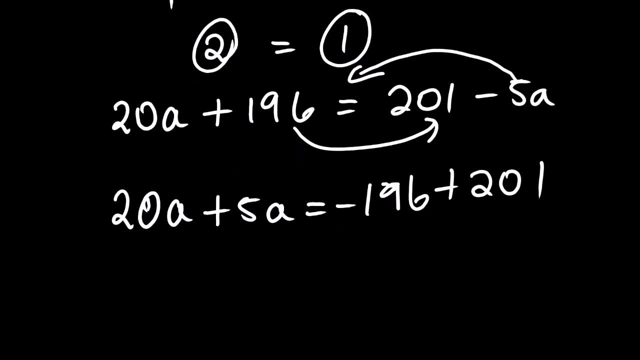 a plus 5a is equals to 1 negative 196 plus 224 этом 1. so 20 a plus 5a is equal to 25 a. so 20 a plus 5 A stay in. it's actually 25k equals to Weburi. 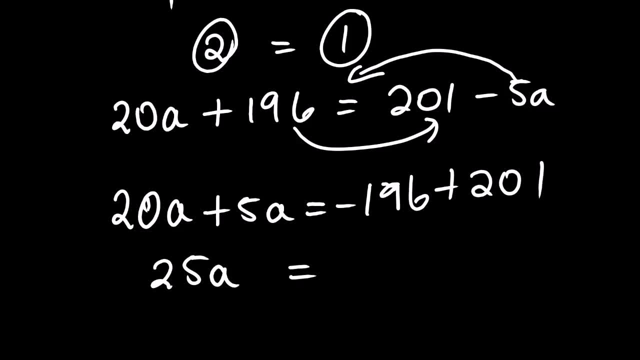 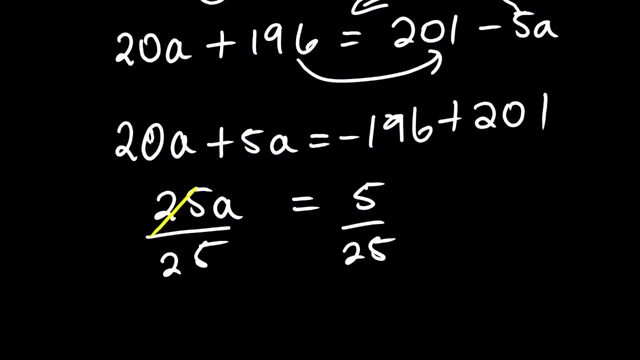 it's equals to 201, minus 196 is equals to 5. then we divide both sides by 25, so this will get rid of this, and then we have a is equals to 0 comma 2 meters per second, so the the system is accelerating upward with 0.2 meters per second. now. 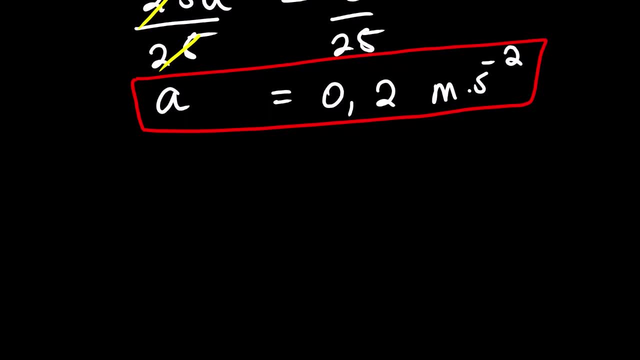 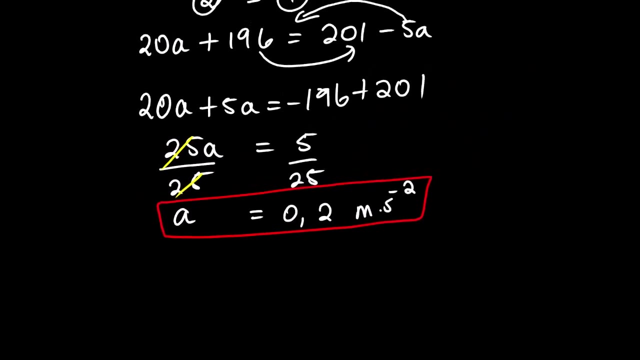 since we have the acceleration, we can quickly calculate our t2. this is actually simultaneous, but in physical sciences, so we can use any equation to calculate our t2. so, looking at this equation, we can calculate our t2. so, looking at this equation, we can calculate our t2. so, looking at this,